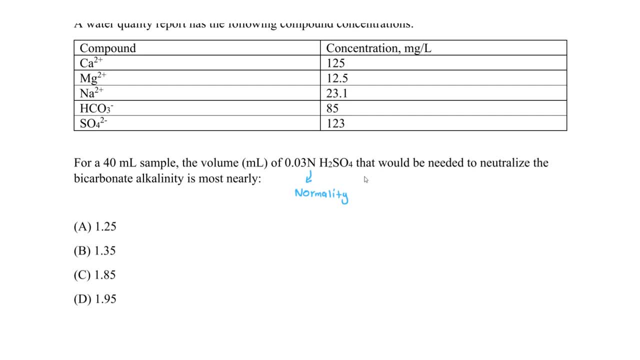 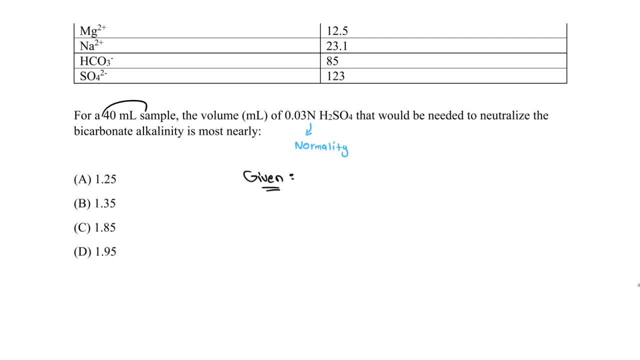 of sulfuric acid at this normality that is needed to neutralize the bicarbonate alkalinity. So if we quickly write what we're given here, we're given that we have this 40 milliliter sample and this, if we draw a picture here. so let's say I have a flask and we have 40. 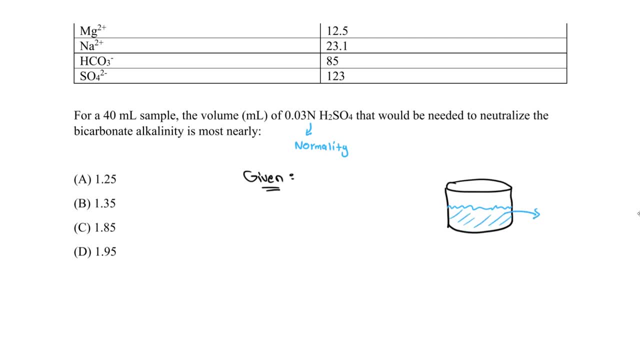 milliliter. So this, and I'll call this. in my solution I use this, So I'm going to call it V1.. I used V1.. I'm just going to call it V1.. And you'll see how this is going to be relevant. 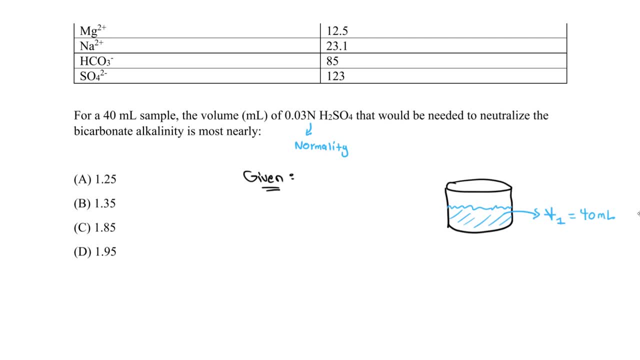 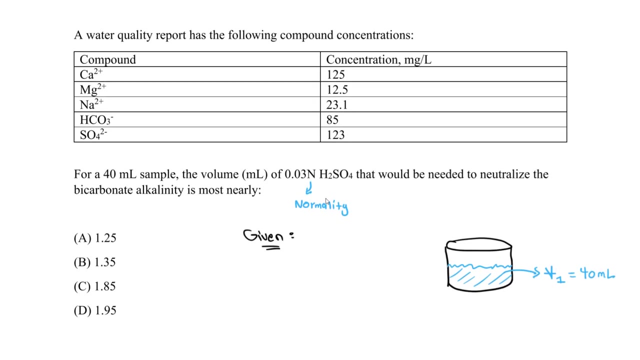 as we proceed and use that equation. So that's the volume of the sample And we're told it has the alkalinity value, right? So this sample is going to have some bicarbonate alkalinity And this bicarbonate alkalinity is given as a concentration here, right? So we're given a lot. 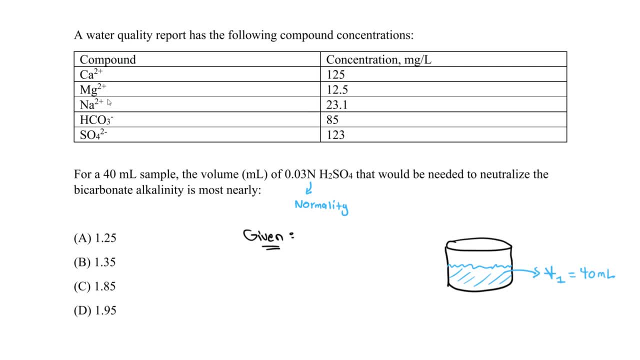 of information. So we have to find the volume of sulfuric acid at this normality And we're going to have to extract what's significant, which is only the 85 here, Because alkalinity, we know it's going to be the bicarbonate ion. If we're determining alkalinity, it's approximation. 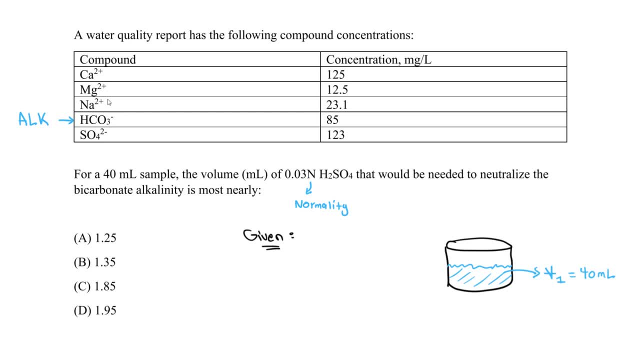 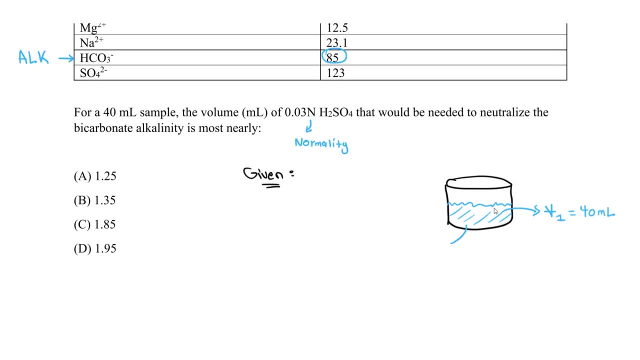 but it's good enough for this example. So we're only using the bicarbonate, always for alkalinity, So we take this value. So we know this sample of water here is going to have an alkalinity value, which is the bicarbonate. 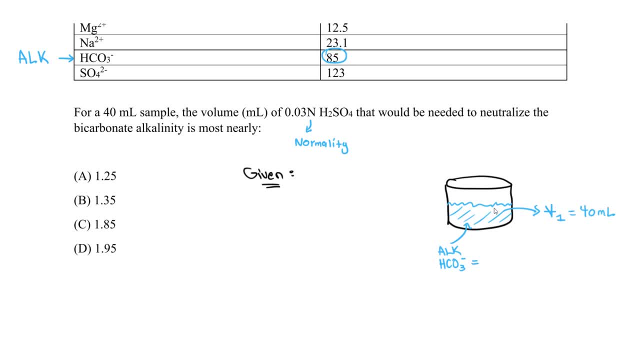 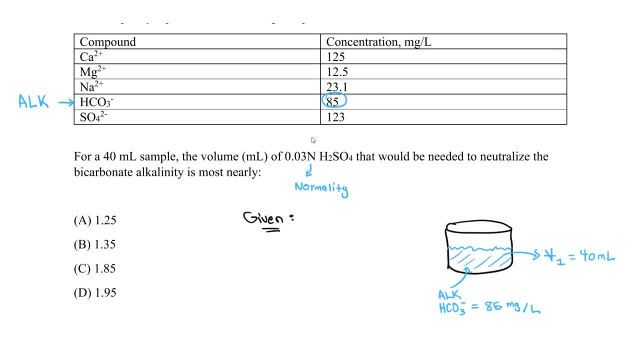 And we're going to have to extract the bicarbonate ion, And it's going to be 85 milligram per liter. Okay, so we have that. And what else do we have? We have the this 0.03 N, right? This is the normality of sulfuric acid. So what we're essentially trying to do is add. 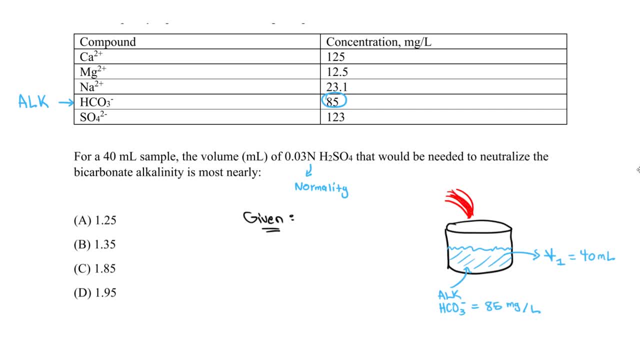 some sulfuric acid. So we're trying to dump a certain amount of sulfuric acid here And we know it has a normality. I'll call the N2, capital N is always normality of 0.03.. And again, this is. 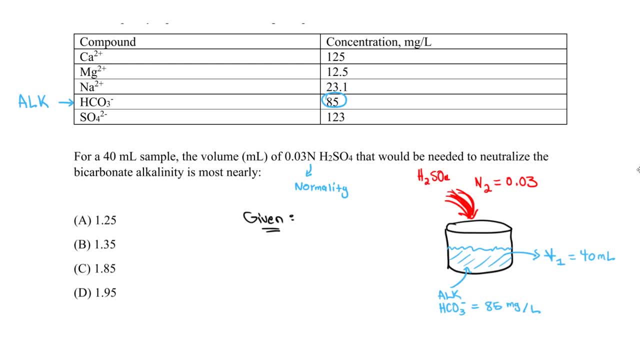 sulfuric acid, H2SO4.. That's what we're trying to add to neutralize the water And specifically for the alkalinity right, the bicarbonate alkalinity. So that's N2, the normality of this. But what? 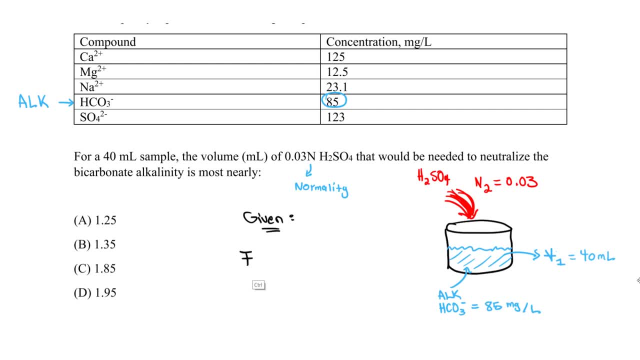 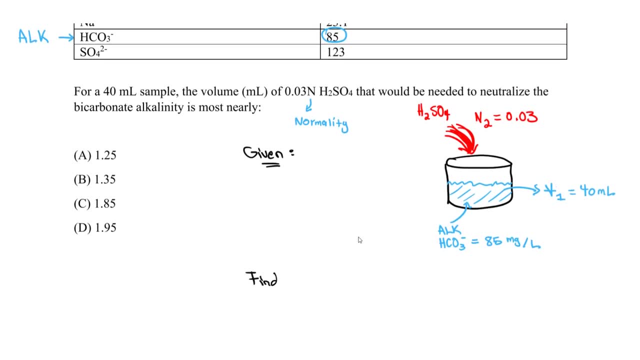 we're trying to find here- let's write this as a fine. So everything here in this figure is a given, And what we want to find is the volume needed for the sulfuric acid, And this is, let's call it, volume 2.. I'm going to say we're going to add some volume 2 here. 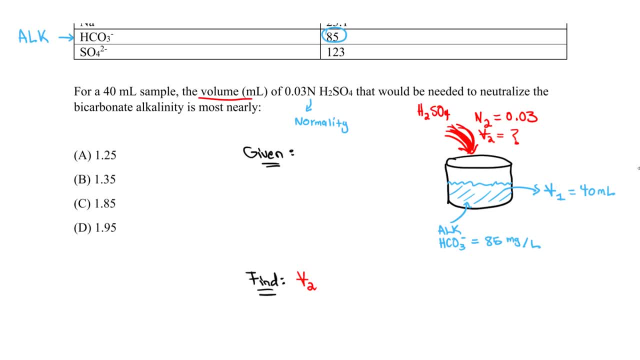 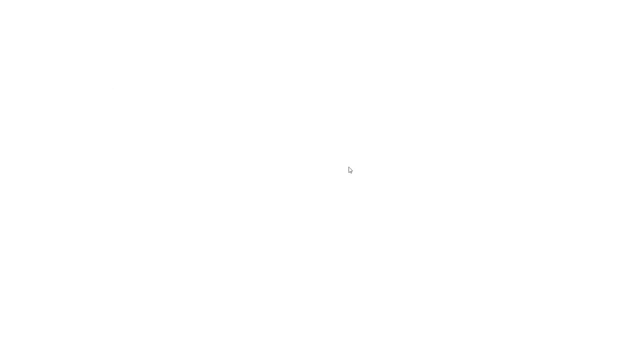 a certain amount, that we want to determine the volume in milliliter ML. That's what we want to find here. So how do we begin? So what I recommend is: first we have to understand that some mallety is a fr FER And 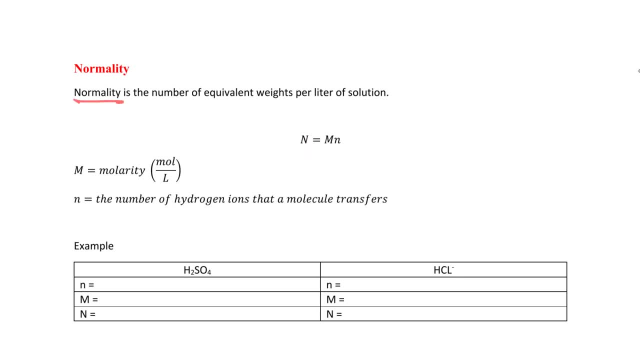 so this is it. We can look meow. confirmation was n bybear 1'. these are my Isso. So Это is going to be the molarity in mole per liter of the specific compound we're looking at right, And n is going to be the number of hydrogen ions. 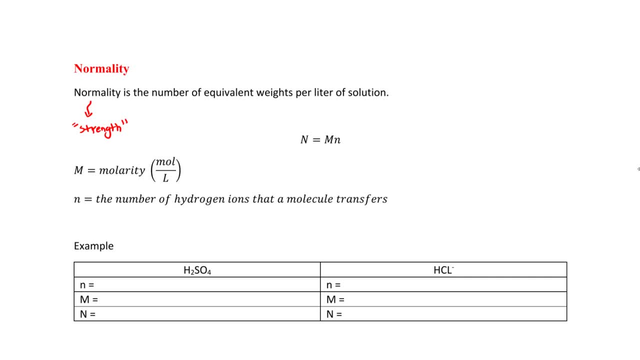 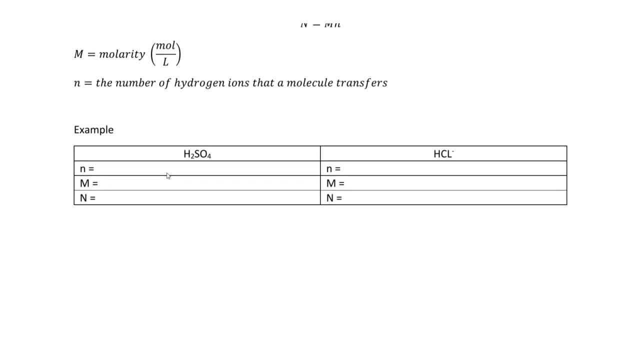 that a molecule transfers. So this n value is the number of hydrogen ions that are transferred in the reaction. So here let's look at two quick examples and compare the two. So on the left side we have sulfuric acid, which is what we're looking at in our question here. 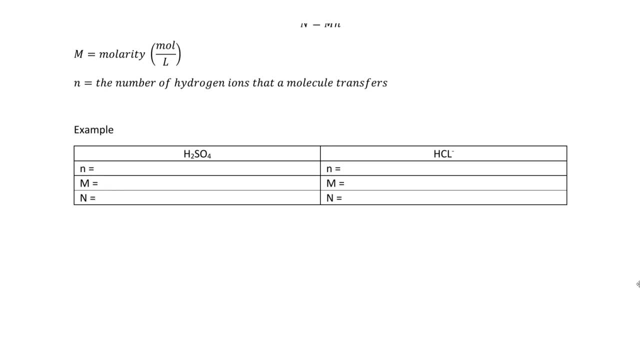 And this is hydrochloric acid. So we know. the n value is the number of hydrogen ions. It's going to be 2, right, We have a 2.. That's the amount that's going to be transferred Capital M. I'm just going to assume 1.. 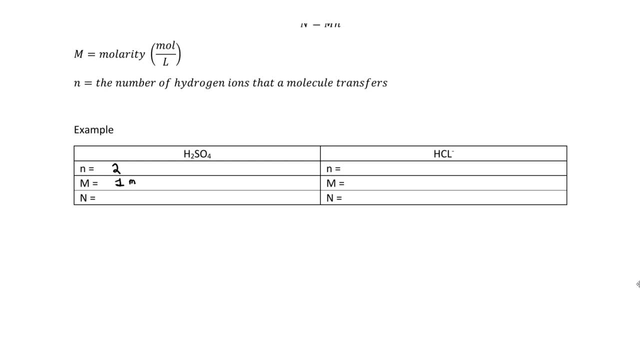 So for each case it's just 1 mole per liter, And for the same here for HCl it's 1 mole per liter And capital N is just going to be m times n, So 2 times 1.. 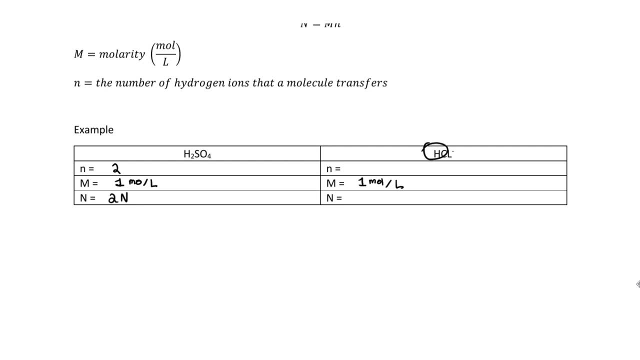 It's just 2n, And this one, the n value here lowercase n, the number of hydrogen ions is going to be 1, right, So there's just one of these. So here, 1 times 1 is just 1n. 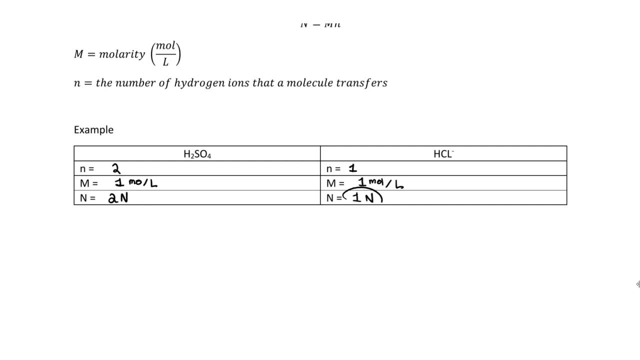 So you can see how the normality here is bigger than this. It's actually 2 times stronger, So it's going to neutralize 2 times better or stronger. So that's what that means: It's 2 times stronger, It's longer than hydrochloric acid. 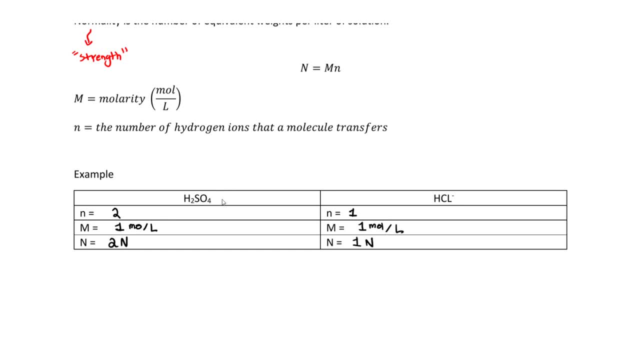 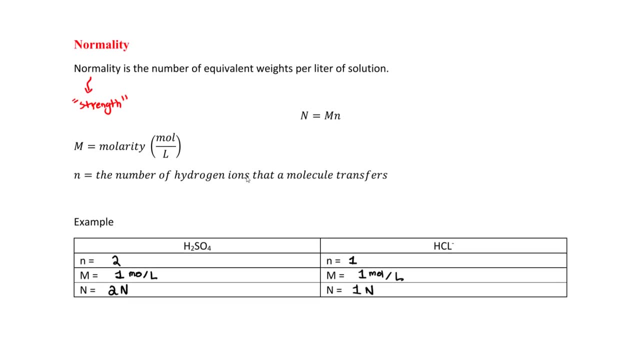 So sulfuric acid has a bigger strength when we're considering neutralization. So that's all that means when we're looking at normality, And the units for normality are going to be equivalent per liter, because this is mole per liter, right? 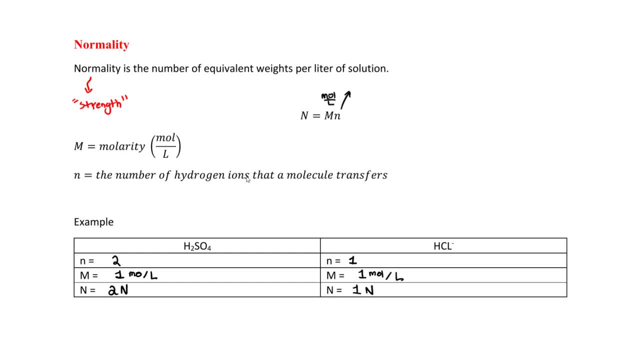 And this n value is specifically equivalent per mole, And if you do the final No units, we're going to get equivalent per liter, And that's our normality. So that's the definition there. I hope that's sufficient enough for us as we do this example. 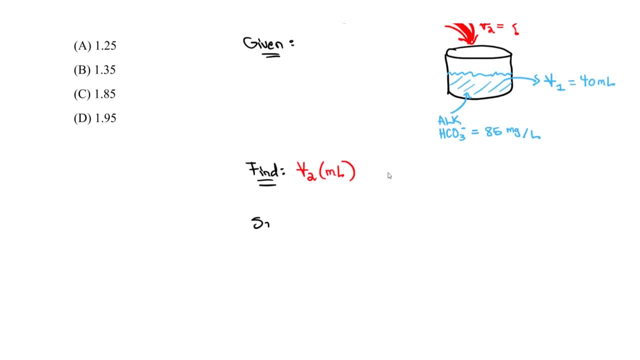 So what do we do next? Now let's write our solution here, And what I'm going to propose is a certain equation, So we know what we can do here is: take Volume 1 times n1,, which is the normality for the water sample. 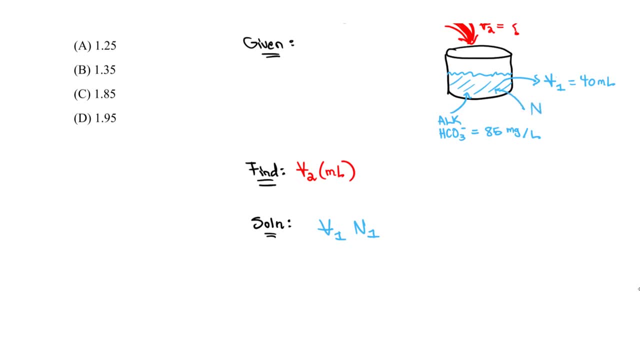 And this water sample is going to have a normality right And it's going to be n1.. But we're not given this. That's why it's going to be tricky And it'll take some time to determine that, So we can find n1.. 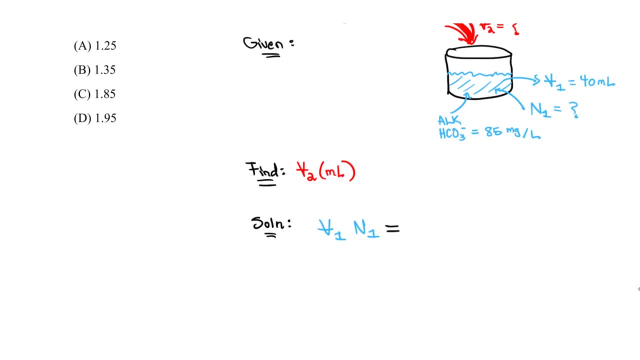 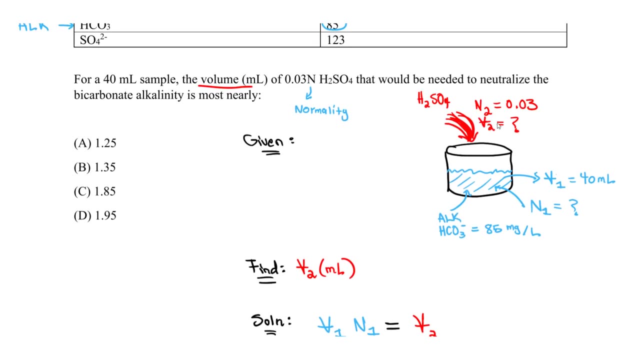 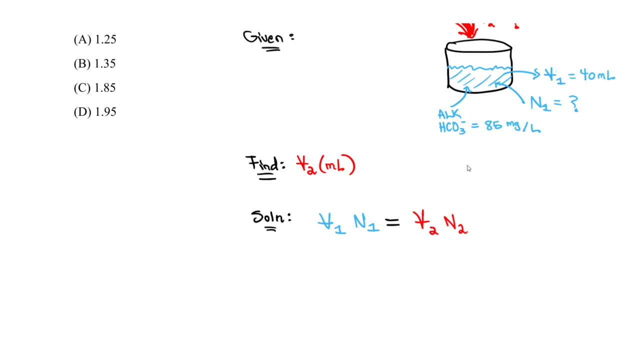 Volume 1, we know, is 40. It's going to equal to volume 2, which is the volume that we need to add For the sulfuric acid right, Volume 2.. And this will be n2.. So you can think of this as the conservation of mass or energy. 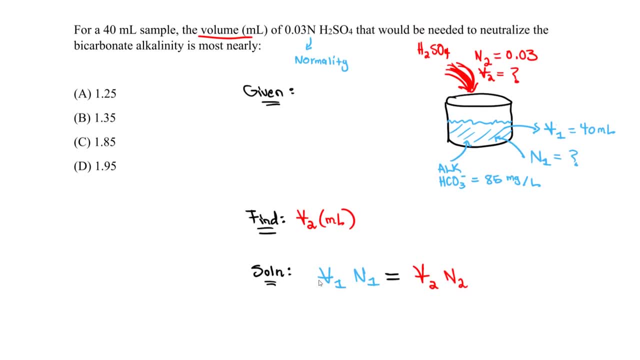 So we know that the water sample is going to have a volume 1, n1. And to completely neutralize this side of the equation we need to input some volume 2, n2.. And n's, here again, are normalities. 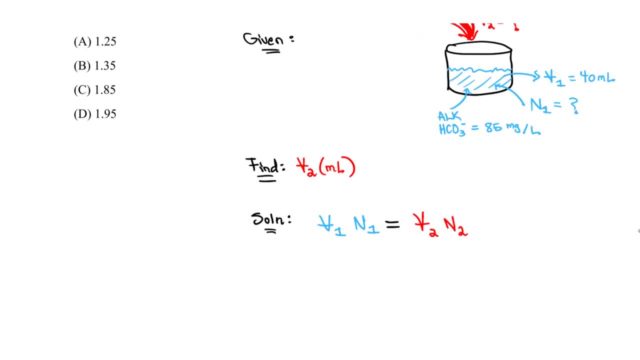 So what do we do now? We know that volume 1 is 40 milliliters. n1: we do not know. Volume 2 is what we want to find. So this is what we want to find in the question And the n2 is given to be 0.03.. 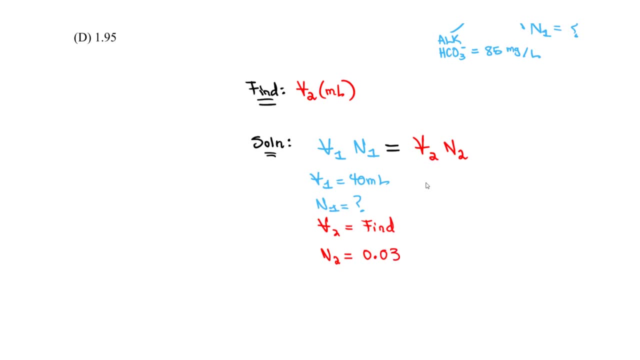 n2, the normality for sulfuric acid is 0.03.. three, So this is essentially the neutralization capacity, or the strength. So now we need to find N one. then we can find V two right, Which is what our goal here. So how do we find N one? So 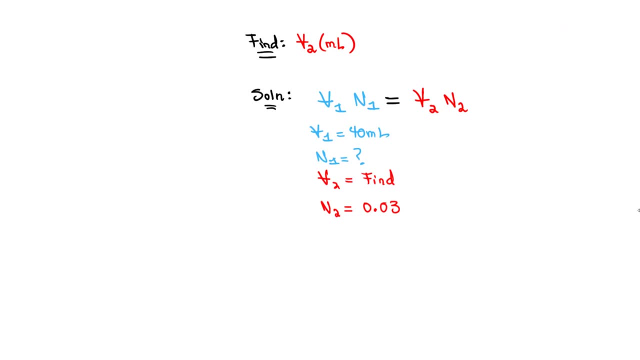 we know again, normality is N times M, So let's write N. one equals N times M. And here be careful here. This is for what? It's, not for sulfuric acid. This is for bicarbonate, right? Because we? 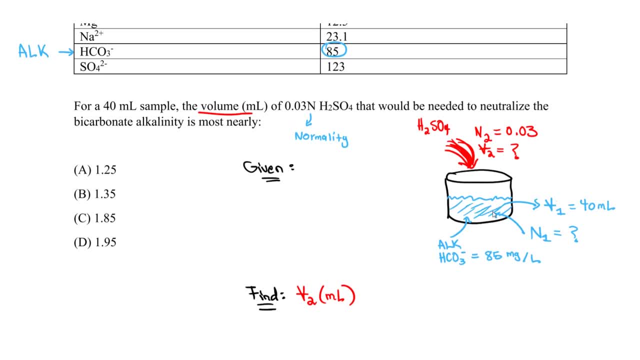 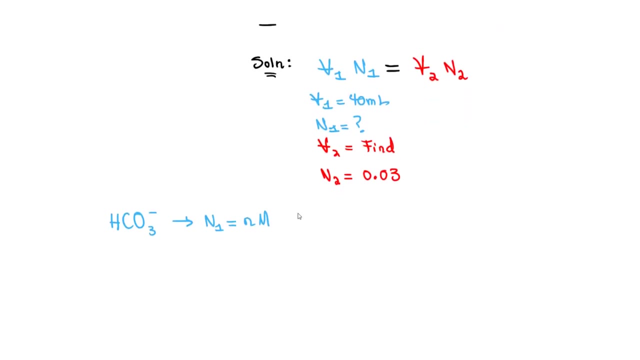 know, the sample here is going to have an alkalinity that we're trying to neutralize- That's what we're focusing on- And it's going to depend on the bicarbonate ion. So what's the lowercase N for bicarbonate? It's just one, right? It's just one hydrogen ion, So it's just one here. So N equals. 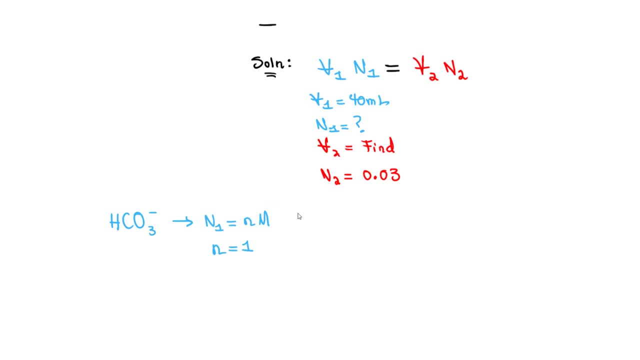 one. And now the tricky part is uppercase M, which is the molarity. But we know for the molarity we're going to need the molecular weight of bicarbonate. So molarity of essentially the bicarbonate ion, which is the alkalinity, is going to equal. it's going to depend on the 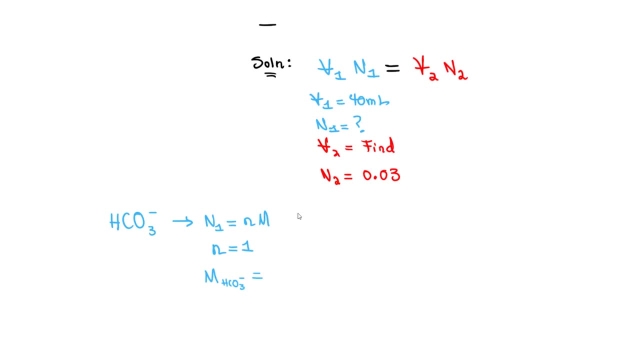 molecular weight. So what we have to take is the alkalinity concentration Times, the molecular weight, And this would make sense when we actually do the units. So what I'm going to do first is find the molecular weight of bicarbonate, And for that we take the atomic 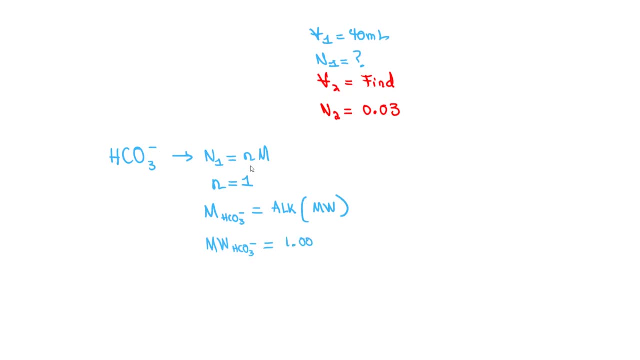 weights. So for hydrogen it's 1.0079.. So this is all in the periodic table. For the carbon it's going to be 12.011 on the periodic table. Then plus we have 3 of oxygen, So 3 times 16.. So for that, if you do the 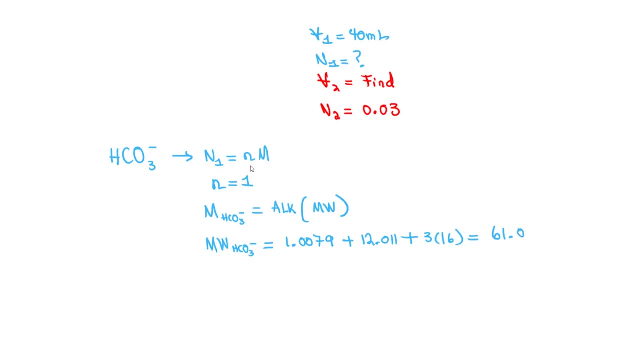 math you should get 61.019 grams per mole. This is the molecular weight for bicarbonate. So we have the molecular weight. What's the alkalinity At the end? we know we want the capital M, which is mole per liter. So we know capital M for. 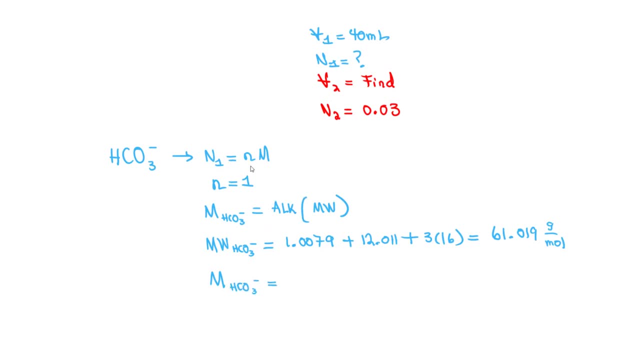 bicarbonate is going to equal to the concentration for the alkalinity, which is going to be the 85 milligrams per liter. So we take 85 milligrams per liter And we multiply by the molecular weight, And this is in grams per mole. So what I'm going to do, 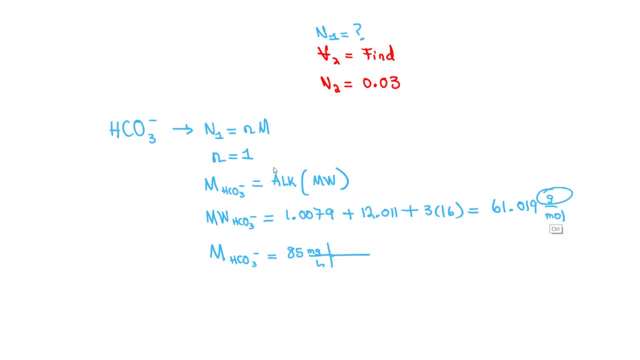 first is convert the milligram to gram, because the molecular weight is in grams. right, So let's convert this, So we have 1,000 and 1 gram. Cancel these out, Then we take the molecular weight. Finally, we plug in here: right, So we take this value and we want. 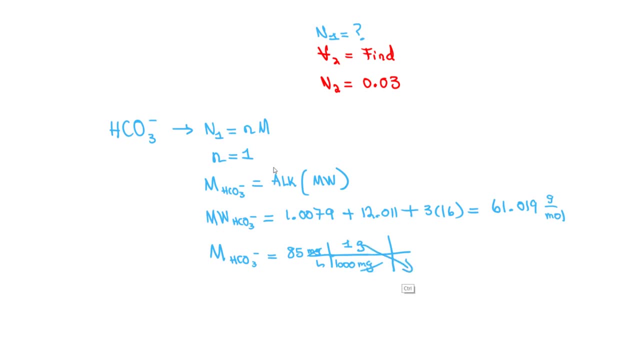 this is on top. Whatever is up must come down, right. So what must come down is this: So it's 61.019 grams. The top is for that per 1 mole. And now we can solve, for the molecular weight of bicarbonate should equal to about 0.00139 mole per liter. That's the correct units, right for molarity. So here we. 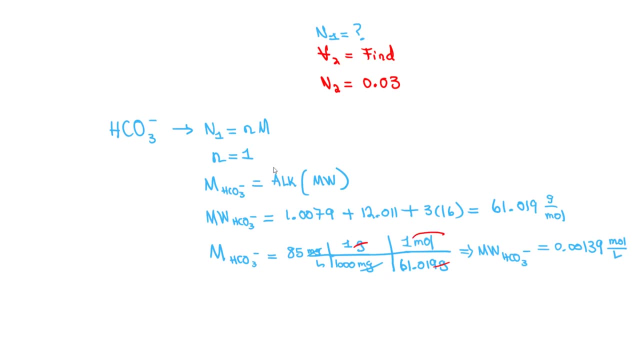 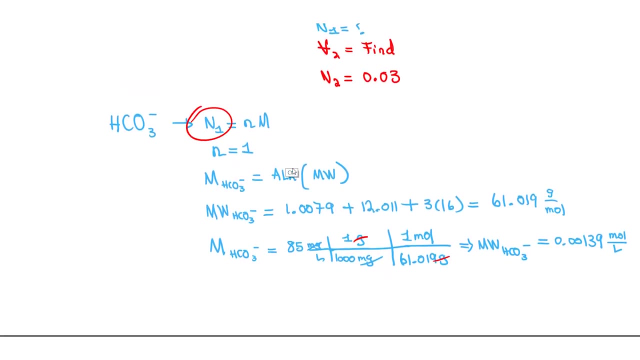 know we did it right. Grams cancel, Milligrams cancel And we have mole per liter at the end. the correct units there. So we have the molecular weight. We're almost done for solving for N1.. So what we have to do here is we know N1 is going to equal to the N value of 1.. And this is that value for N. And we multiply that by the molecular weight of bicarbonate, which depends on the alkalinity. Essentially it's our alkalinity there And we multiply it by this right. So here N1 is equal to the N value of 1.. And we multiply that by the molecular weight of bicarbonate, which depends on the alkalinity. Essentially it's our alkalinity there And we multiply it by this right. So here N1 is equal to the N value of 1. And we multiply that by the molecular weight of bicarbonate, which depends on the alkalinity. Essentially it's our alkalinity there And we multiply it by this right. So here N1 is equal to the N value of 1.. And we multiply that by the molecular weight of bicarbonate, which depends on the alkalinity. Essentially it's our alkalinity there. And 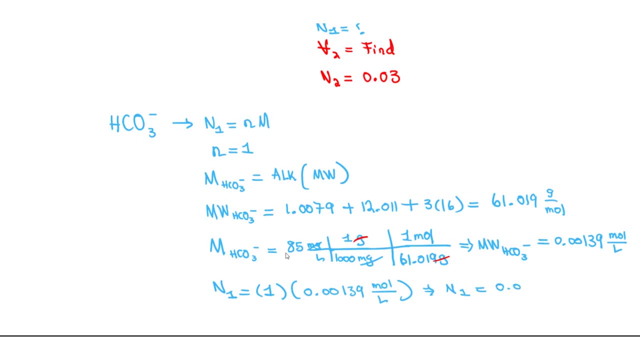 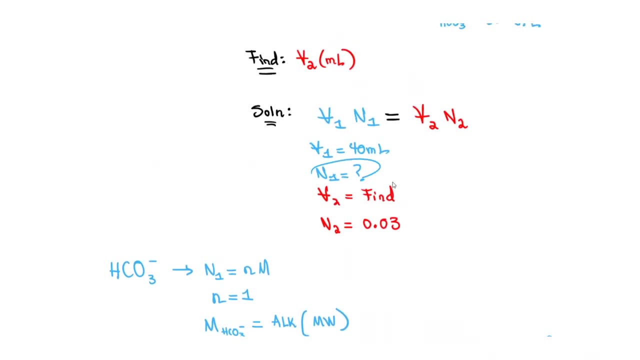 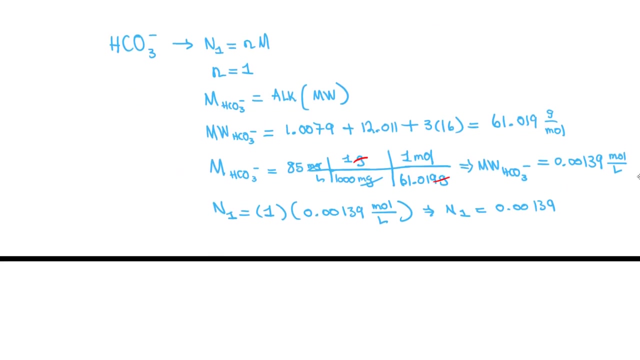 1 is going to equal to just that value. So we have our N1.. And it's going to be this. Then we can just solve for V2, right, The total sulfuric acid we need. So I'll just do it down here. So what we're going to say is: V1- N1 equals to b2. 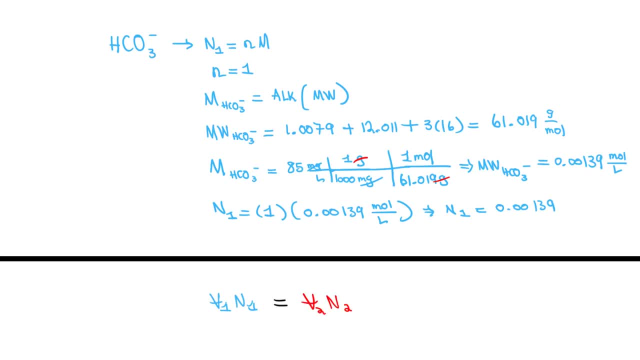 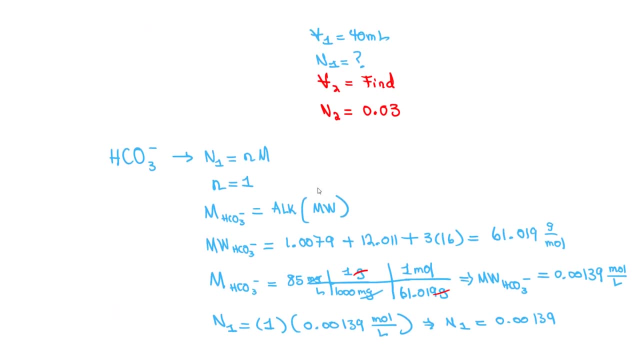 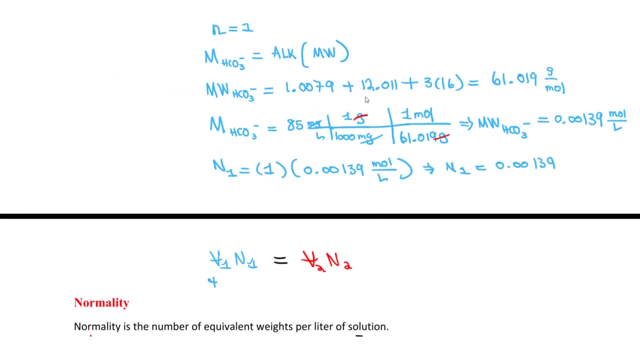 N2.. So here we know. so running out of room, but V1 is given above to be the 40. And we found N1, right, It's this value. So V1 is 40 milliliter, N1 is 0.00139.. And this is. 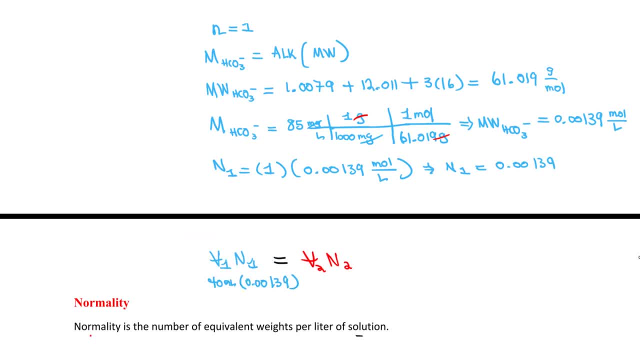 specifically for bicarbonate, right, Because we're focusing on alkaline, on neutralizing alkalinity, And we know this is V2.. V2 is what we want to find the total sulfuric acid we need to add to neutralize that bicarbonate. alkalinity And N2 for sulfuric acid, the 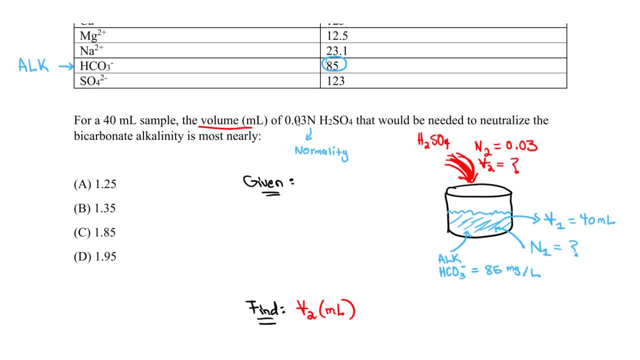 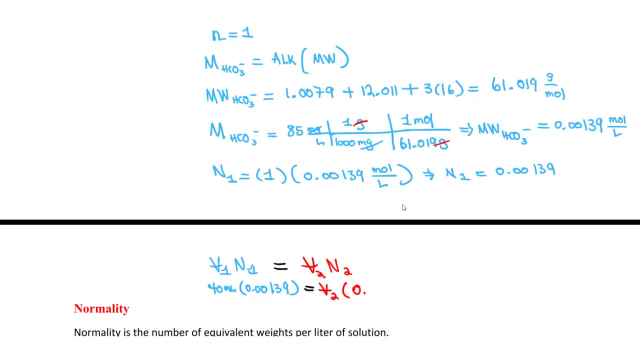 normality is what It's given here: 0.03.. I wrote it here and I wrote it here, So 0.03.. So now? So now all we have to do is solve for V2.. And for V2, the total sulfuric acid we need is about.